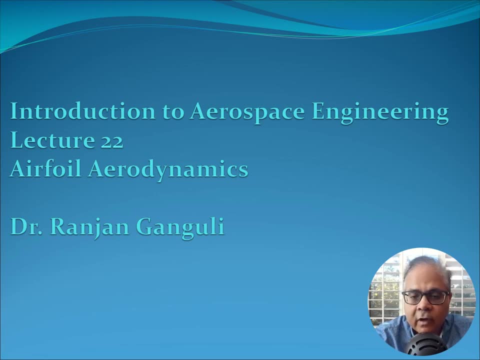 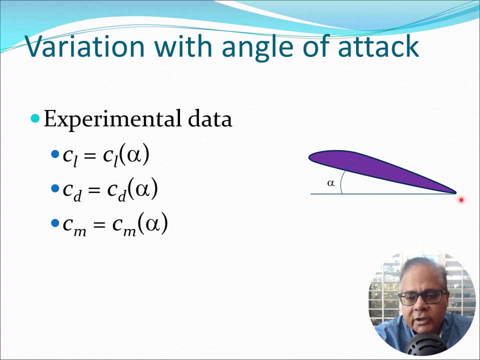 respect to alpha, which is the angle of attack which the airfoil section sees with respect to the flow. I am Dr Anjan Ganguly. Now, if we look at any airfoil section, we have already seen that the lift drag and pitching moment characteristics can be. 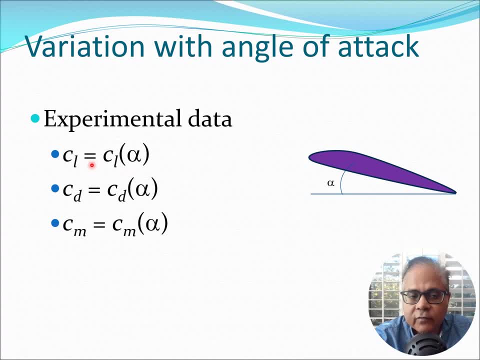 summarized through certain coefficients which are the lift coefficient CL, the drag coefficient CD and the moment coefficient CM, and these are essentially functions of alpha, where alpha is the angle of attack. So if we look at the airfoil section, we have already seen that the 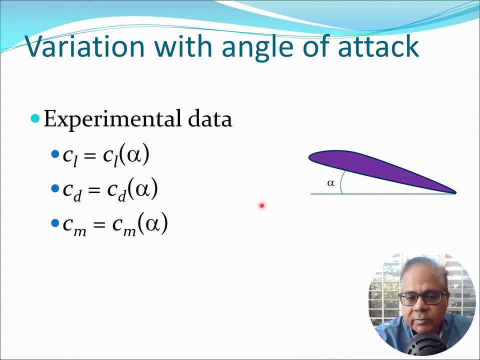 airfoil section is an angle which the airfoil chord line makes with respect to the airflow. So I am assuming the airflow is coming along this particular line here. So, as you will expect that if alpha goes up these values may change and so on. So how do we obtain this relationship Now? 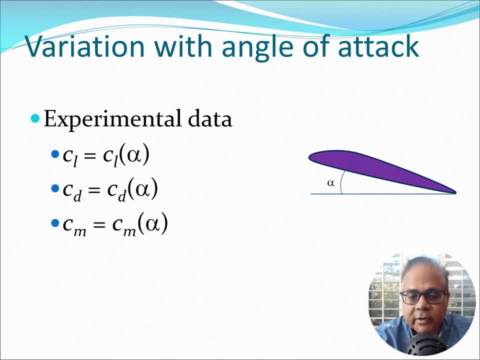 one of the ways is, of course, to use experiments here. Experiments are always the truth figure as far as any physical system is concerned. So we are going to look at the airfoil section concerned. so that's the way to go about it. 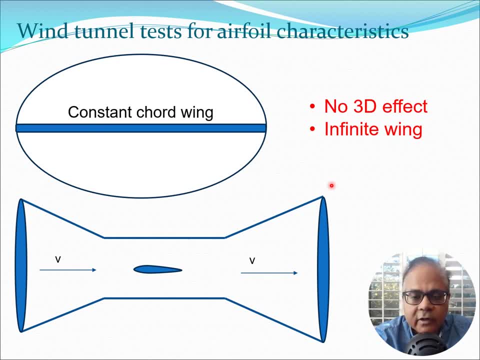 So whenever we are thinking of any airfoil cross-section, we are essentially assuming what is known as an infinite wing. So what happens in an actual wing is that there is some flow from below the wing to the top of the wing, and so this constitutes what is known as a three-dimensional effect. 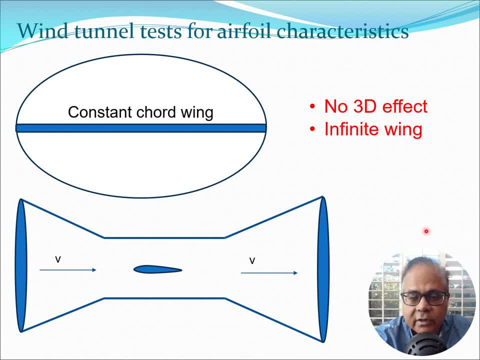 Now what happens in an airfoil section is that we are considering a two-dimensional wing and therefore there is no such flow taking place. So what we do is that we make a wing such that it spans from one end of the wind tunnel to the second end, and this is a constant chord wing. 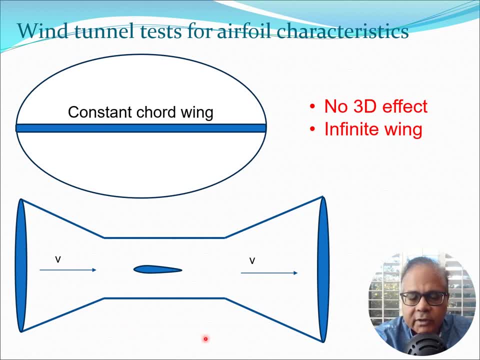 So this is the front view of the wind tunnel and this is the typical side view. So essentially, the air is going in here, we have the cross-section somewhere in the middle and then, toward the exit, The air is again going out. I have just given these schematically. 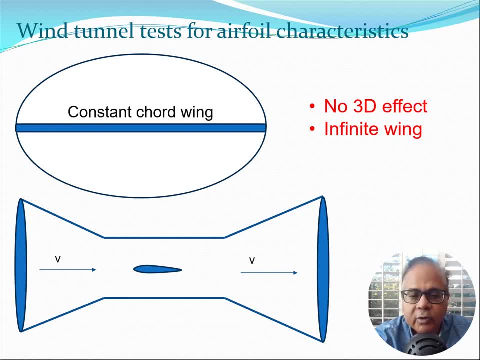 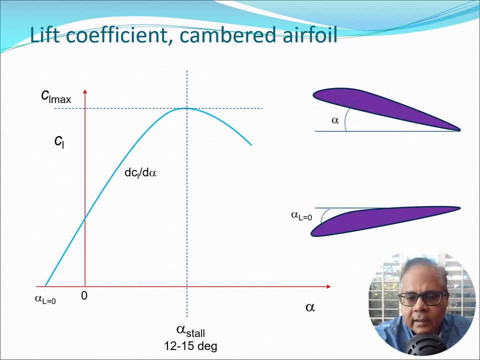 These velocities are, of course, going to be different, governed by continuity equation and Bernoulli equation, as we have discussed in some of our previous lectures. So when we do these tests, what do we obtain? So let's start with the lift coefficient for a typical cambered airfoil and in that case, 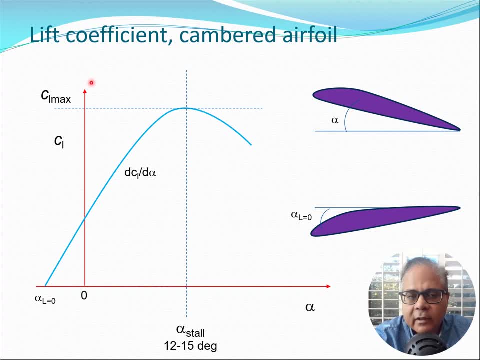 the CL versus alpha curve is like this. So I have given it by the blue line, I have given it by the blue line here. So there is a linear region till a point and then the CL value starts going down or the lift starts going down. 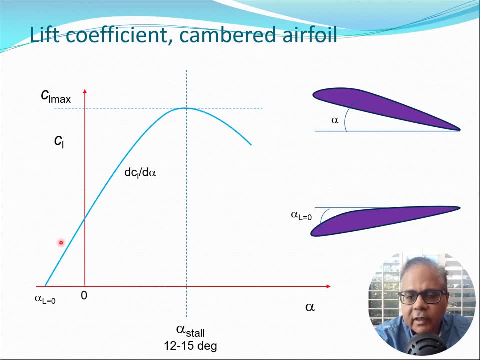 So what we do is that we very often in our calculations consider only this linear region, and this point where the lift starts going down is essentially related to stall, and stall is related to flow separation. So this alpha stall value could be something like 12.5.. 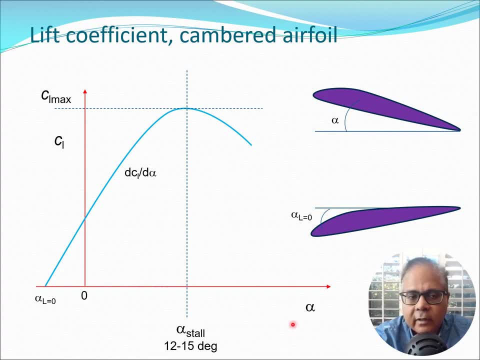 So this is the flow separation. This is something like 12 to 15 degrees for many airfoil cross sections. Now the maximum value of lift here is known as CL max and there is a value here, alpha L equal to zero, which is actually the CL value being zero and the alpha corresponding to 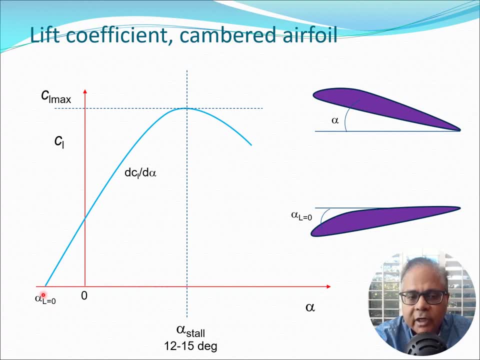 it. So this is going to happen whenever there is a cambered airfoil present, because what happens in the cambered airfoil is that, even if you put it at zero angle, There is going to be some lift generated there, and so you have to put it at a slightly negative. 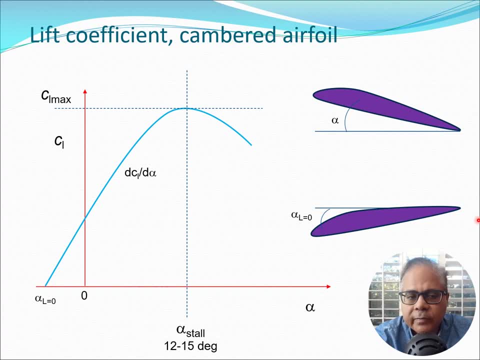 angle here, so that the lift essentially becomes zero, which is this point here. At this particular angle, you can see that CL has reached the zero point. Now, of course, you can clearly see that the slope of this lift curve is DCL by D, alpha. 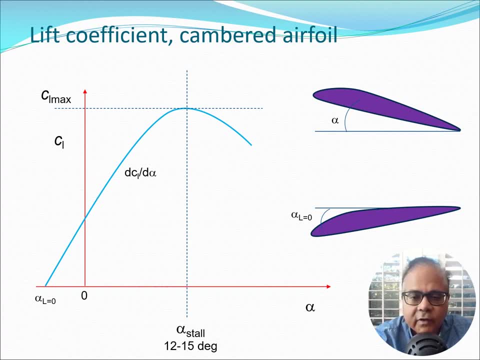 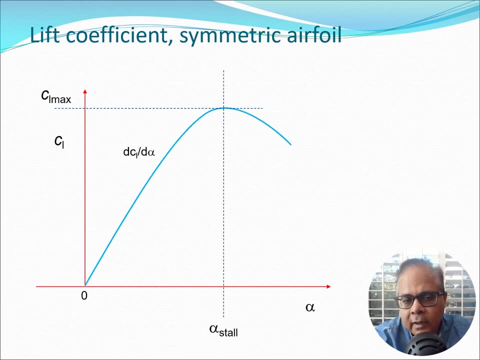 This is a very important parameter which often figures various issues in the practically linear equations equation. So this is often known as the lift curve slope. Now, what would happen if we had a symmetric airfoil? If we had a symmetric airfoil, the curve would essentially pass through. 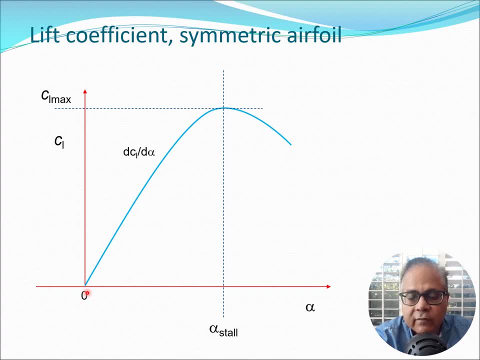 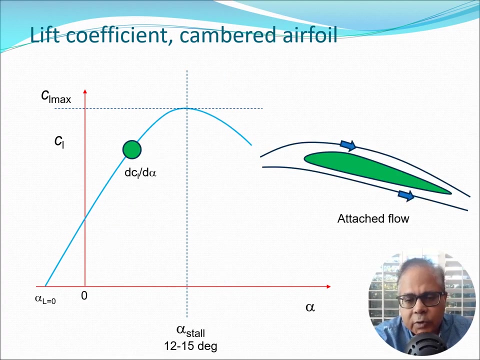 zero. So when alpha would be zero, CL would be zero. And there are many situations where symmetric airfoils are used. For example, as far as helicopter rotors are concerned, symmetric airfoils are quite ubiquitous. So let us now look at the physics at two different points in the 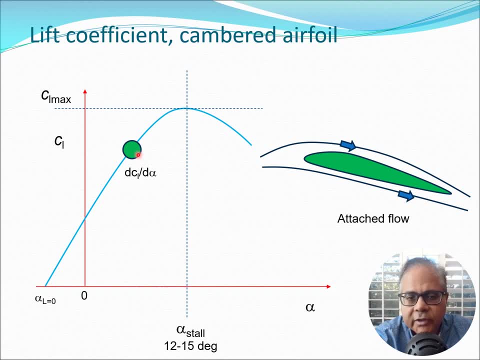 flow. So first let me start with this point I've shown in green here. This is a point in the linear unstalled region, which is the nice looking region given by the straight line. Now this region corresponds to essentially attached flow around the airfoil cross section. So you have a typical. 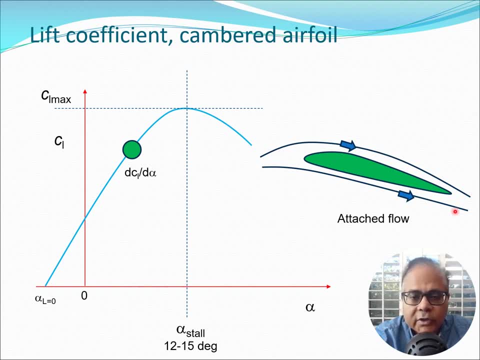 airfoil here. So you have a typical airfoil here. You have the streamlines which are going smoothly around this airfoil cross section. This is the typical flow we like to have And this is the flow at which often cruise takes place for most. 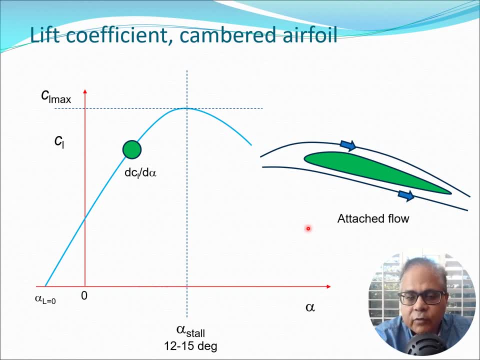 aircraft which are flying in passenger flight. For example, if you are traveling between any two cities in a passenger jet, you are likely to be cruising at a very low angle, such as five degrees or something like that, And so the flow is going to be attached here. 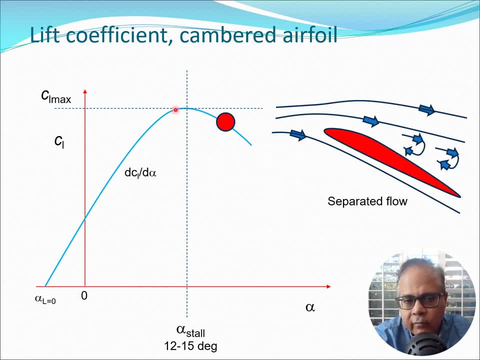 in general. Now, what about the situation here, which I have shown in red, And here you can see that the lift has started to fall. So this is actually in the stalled region. So after alpha stall, essentially there is flow separation And so therefore the lift has started to decrease. 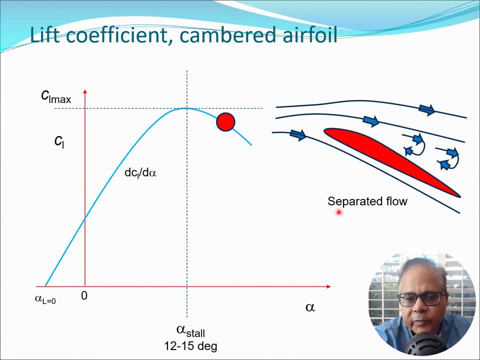 So in this case the airfoil is like this. the angle is more you can see here. it may be 17 degrees or something like that, And in that case you can see that the airfoil is going to fall. So 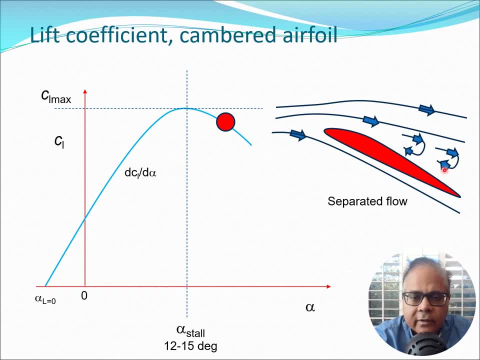 you can see that there is separated flow in the region which is near the trailing edge at the upper surface, And so this is, of course, call related to the boundary layer getting separated and so on, transition from laminar to turbulent and all those different phenomena which we 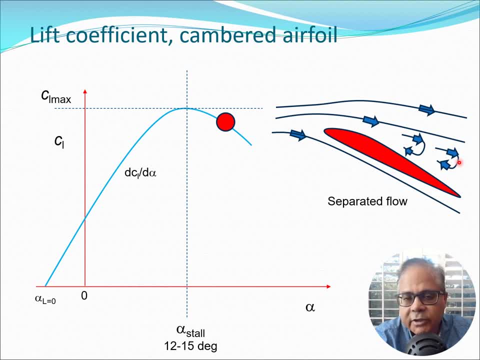 discussed previously in the video related to flow separation. So, essentially, keep in mind that most of the airplanes actually try to fly in this regime, which is the linear regime, because that's where you get nice characteristics as far as the airflow is concerned and you get a. 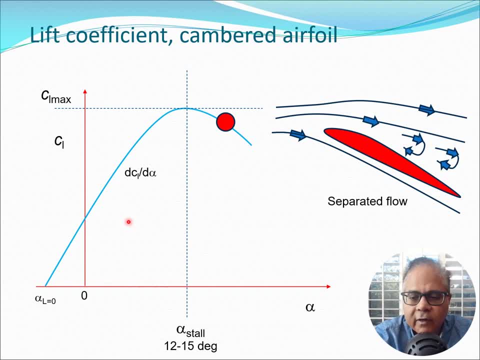 increase in CL with any increase in alpha. Now, once you are in this region, any increase in alpha is actually going to lead to a decrease in CL, which is not necessarily good for the pilot in terms of controlling the aircraft and in terms of generating enough lift to keep the aircraft in. 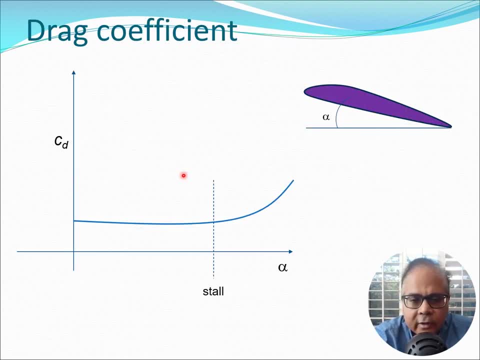 air. So now let's look at the different coefficients, the drag and the moment. So first let's look at the drag coefficient, which is CD. So CD has actually somewhat like this: it's more or less constant, And then it. 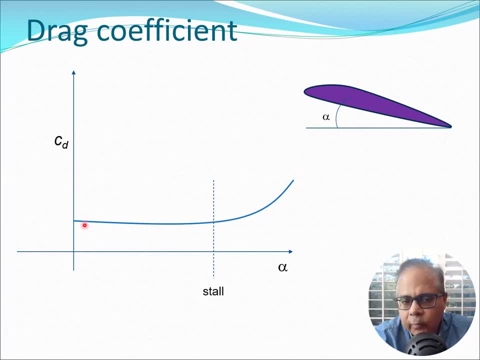 starts going up after stall at this point. Now this is not really constant, But in many cases people do assume CD to be some constant value, CD zero. But actually there are some models which tell you it's kind of like a quadratic polynomial. So we'll look at some of the math models. 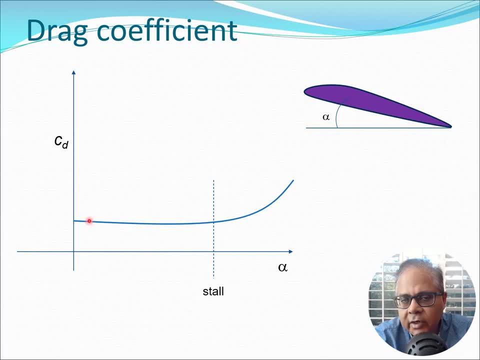 later. So again, of course, remember that drag is always positive because we are living in the real world, there is friction, there is viscosity And therefore CD value is always going to be a positive number. CD is all, is always going to be on this side of the graph. Now, next is the moment. 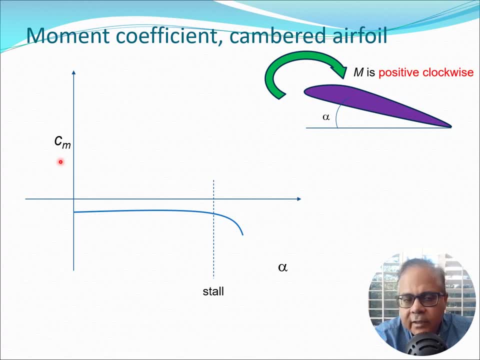 coefficient, cm. And before we discuss the moment coefficient, let us define the typical notation used as far as moments are concerned. So if we have the airfoil section, moment is positive clockwise. So that's the direction I have shown here. So now what happens is that if you have a 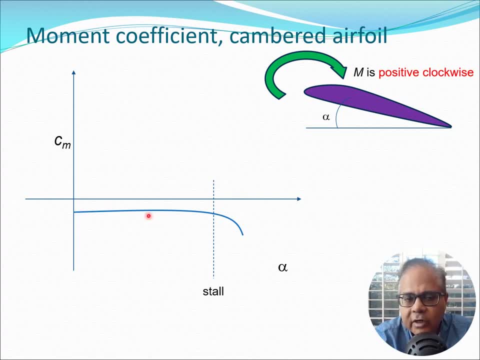 cambered airfoil. the moment is actually a small negative number, And so it's somewhat like this. And then, after stall, of course, there is a sudden change or fall. in the moment, here there are large torsional loads which can actually be generated because of this. 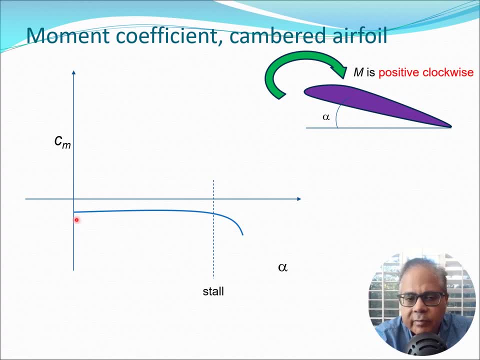 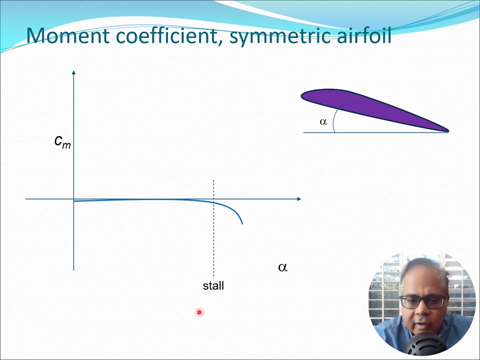 So if you have a cambered airfoil, you can actually get a small fall in moment, and which can be quite drastic. But keep in mind that, like I mentioned before, most of the airplanes try to work in this region, And so here the moment is somewhat of a constant, though it changes to some extent Now. 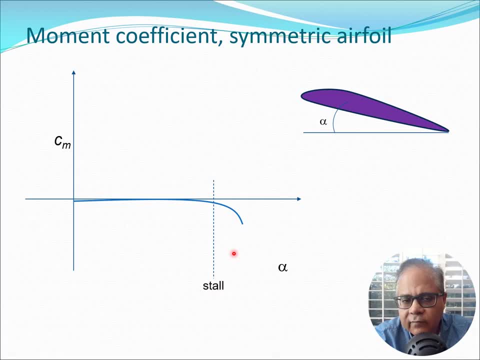 if you were a symmetric airfoil, then your moment would be something like this. So essentially it would be quite small or nearly zero, and then it would be something like this. So this is one of the reasons why, in certain situations, we actually use 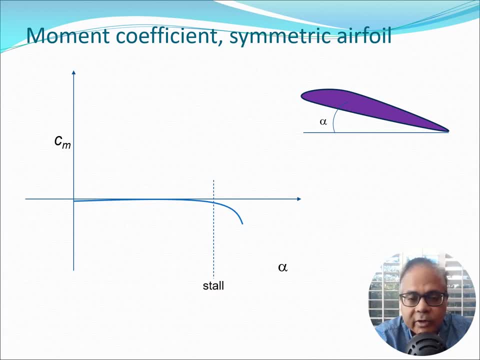 the symmetric airfoil, because we don't want moment generations to take place, because moment, like I mentioned before, can lead to torsional loads or twisting type of loads being generated on the wing section or on the rotor blade if you are in a helicopter. So now let's turn to the math model. 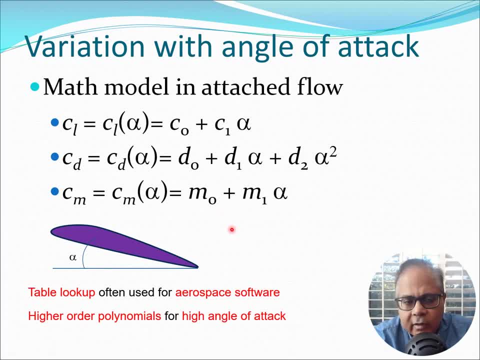 model. So let's look at some of these phenomena. And these are all in the region below the stall condition, So essentially these are in the attached flow region. So CL can be expressed as C0 plus C1 alpha, where C0 and C1 are constants, And you can obtain these constants from any experimental data by essentially 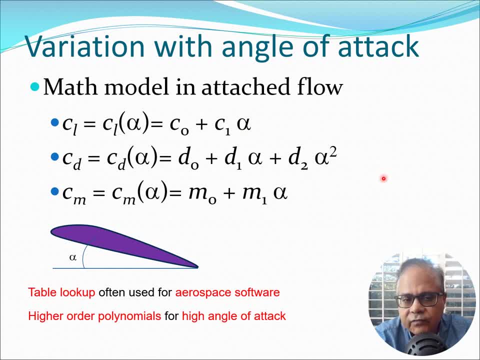 fitting in this kind of a straight line to it. CD can be expressed in this form here: D0 plus D1 alpha plus D2 alpha square, And CM is M0 plus M1 alpha. Now, these simple models are very often used in many situations. For example, if you are 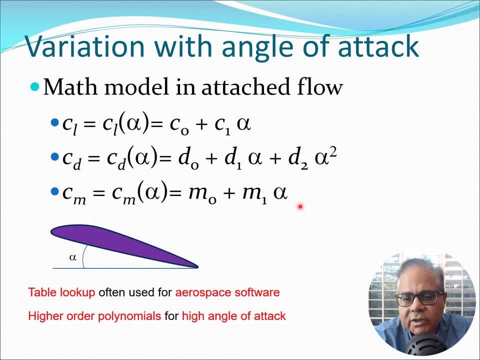 trying to derive certain expressions in terms of CL, CD, CM. at the end of those derivations we often put in these equations here and then we put in the values of alpha correspondingly. Now do remember that in reality things are. 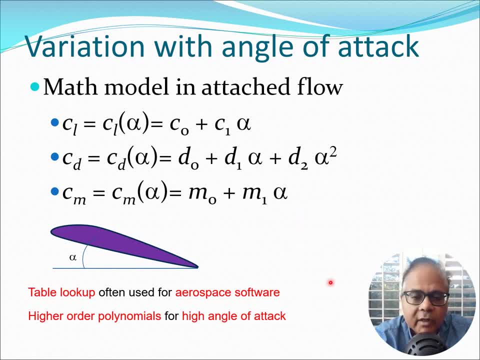 more complex Here. we have assumed that the Reynolds number and the Mach number are essentially at certain fixed values. But in many cases you may actually have to consider the fact that Mach number and all number are also changing And you can use a table lookup type of situation there where you have 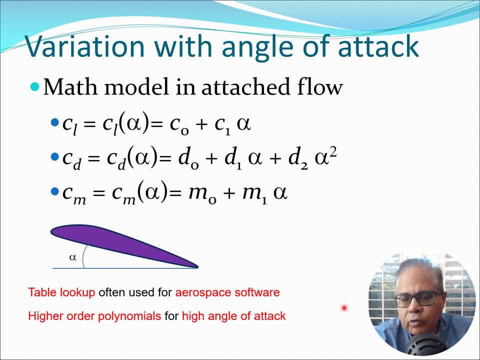 values of these different parameters And you can simply go to the curve or the table and get the corresponding values. So there are two options here: you can use table lookup or you can use polynomial fits on the data which you have obtained from any kind of internal 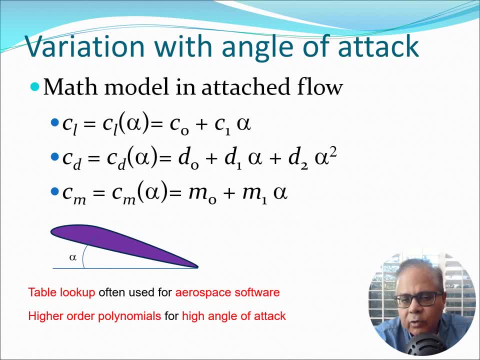 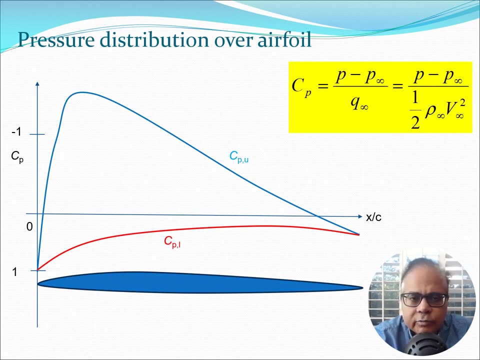 experiments. Now I find that most people prefer table lookups because it is very easy to do an interpolation and to find out the CL, CD, CM value corresponding to any particular alpha value. Now let us look at the pressure distribution on the airfoil. 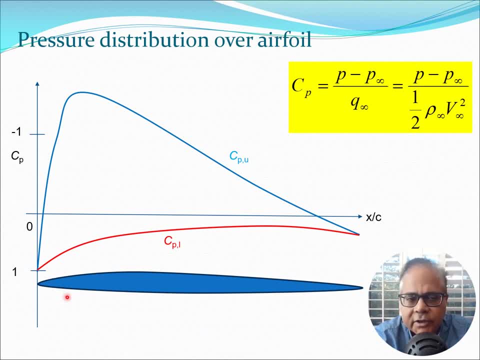 So again contemplate this kind of airfoil section here. So we had already defined CP in a previous lecture And just to review it, CP is P minus P infinity, So this P is Q is Q infinity per v. So Q is Q infinity by Q infinity, where Q infinity is the dynamic pressure, half rho infinity. 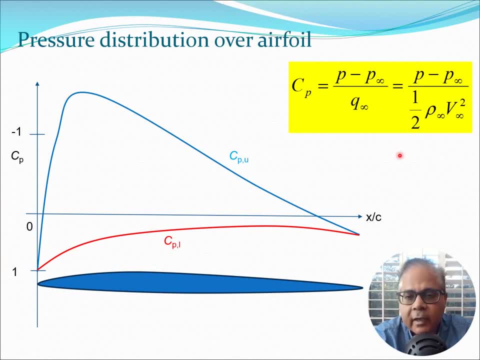 v, infinity square, and infinity refers to the freestream value, So it is the air coming from front And of course rho is density, v is velocity of that freestream air and P is the pressure on the surface of the airfoil. So if we plot the pressure for the 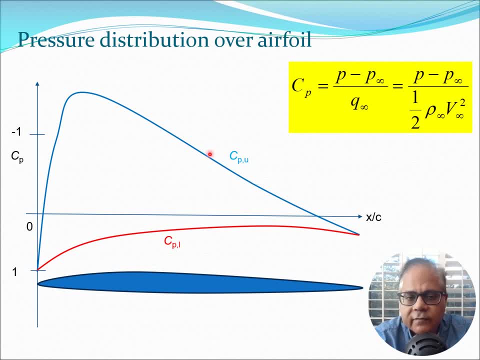 lower surface. we get this red line here. start the pressure for the upper surface. we get this blue line here and on the top and the pressure which is coming from the upper surface, that is a suction pressure. So there is a negative value here of Cp minus 1 and here it is Cp1.. 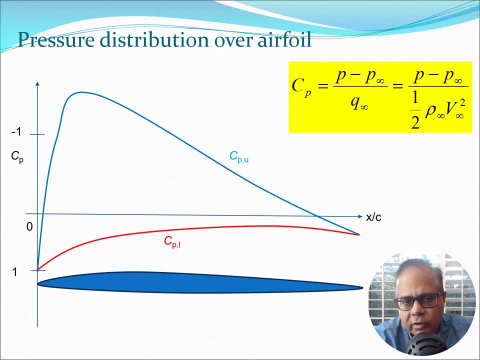 Now this particular graph tells you a lot about the pressure which is essentially generated by the airfoil, and one of the reasons the airfoil selection is very important and often ubiquitous as far as aerospace engineering is concerned is because airfoils give you very attractive pressure distribution. 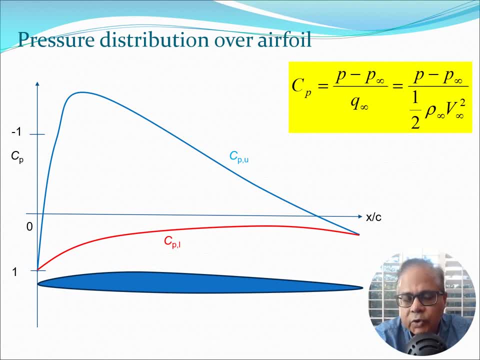 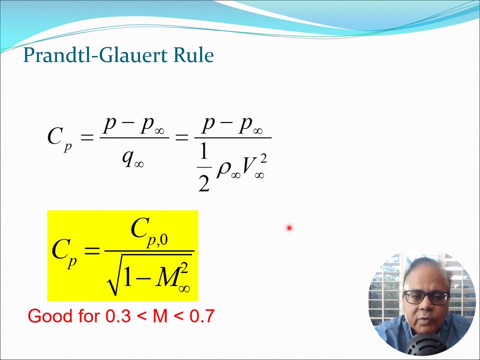 As you can see, there is a very good suction at the top, and so you get very good lift to drag ratios, and these are very attractive features for aerospace engineers. Now, one more thing to remember is the Prandtl-Clauerts rule and Prandtl-Clauerts rule essentially 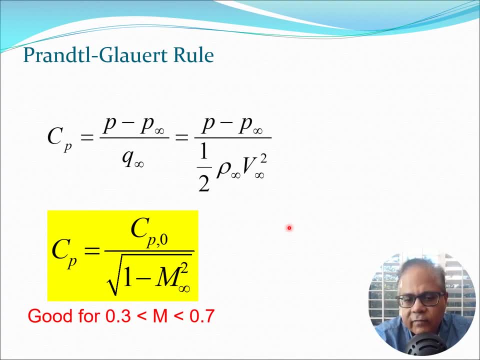 lets you modify the Cp value to include the effect of compression. Basically, we can modify the Cp value between 0.3 and 0.7. so remember you are using the Prandtl-Clauerts rule for many calculations in very simple and quick way. 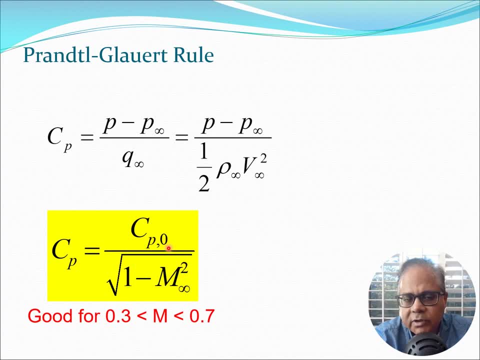 So in the next slide, I will tell you the Prandtl-Clauerts rule. So this is the Prandtl-Clauerts rule. Now, in the next slide, I will tell you the Prandtl-Clauerts rule, which is essentially. 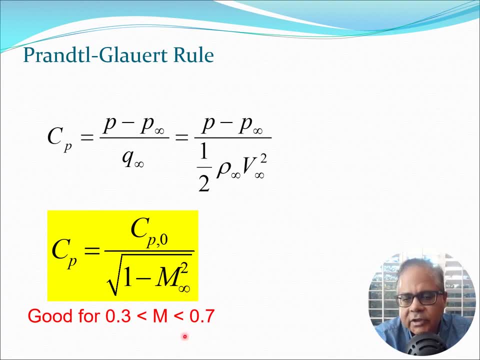 that the airfoil splitter has a expression for the airfoil that is going in this direction. that means that the airfoil is moving in the direction that the airfoil is moving in the direction that the airfoil is moving in. So the Prandtl-Clauerts rules happen at the point where airfoil으s is being generated. 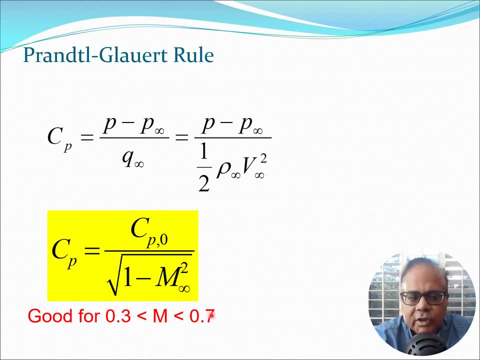 by other airfoil and their own airfoils are getting the airfoil flow in incompressible flow. So in this region you can pretty well use the Prandtl-Klauert rule for many calculation. Do remember that if you are more than 0.7, this rule again. 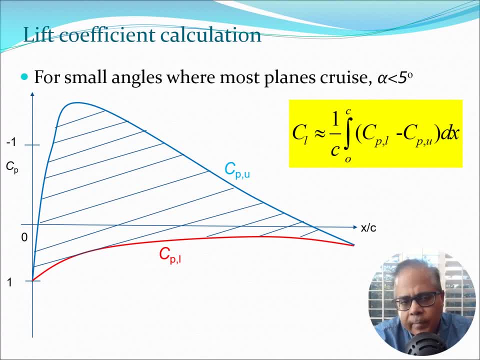 starts breaking down. Now how would you calculate the lift coefficient from the Cp value? So, like I mentioned, if you were to do an experiment in the wind tunnel, you could use pressure sensors to get this kind of curve for Cpu and Cpl And we can actually relate Cl to Cpl and Cpu. 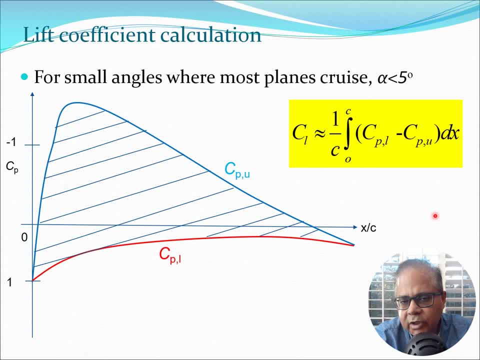 in this manner here. So essentially, as you can understand, it is the integral. So if we go from the front to the end of the airfoil, what we have to do is to integrate this and subtract this. So, essentially, what this integral is telling you mathematically is to find this cross section. 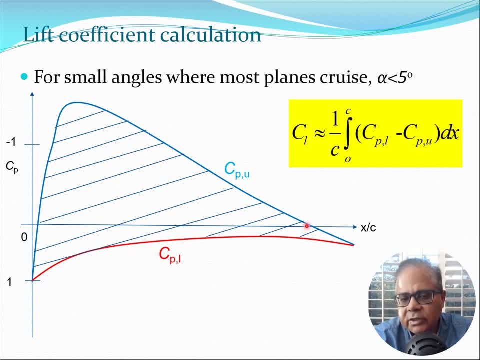 which I have. So that is shown in these dash, in these lines here. So essentially, whatever is inside this particular Cpl-Cpu curve is going to be Cl. Now this expression is actually derived from the fact that there is a normal force constituent from Cp, And so that is the source of the lift And it is. 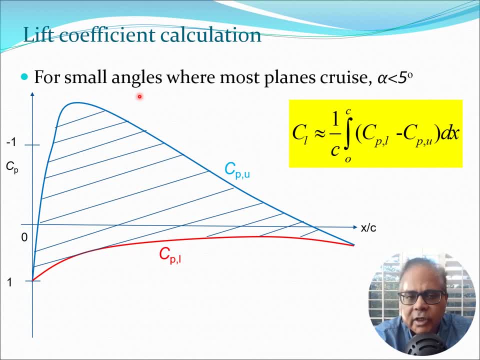 valid for angles which are small, So, fortunately, most planes fly at relatively small angles, such as a alpha is less than five degree. This is where most airplanes cruise, And so therefore, we can use this expression to immediately get Cl for our particular problem. Now, just like I mentioned for 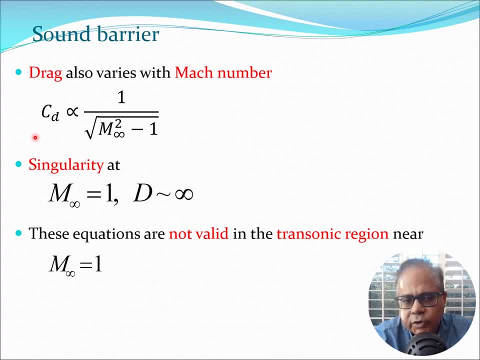 Cp. there is a fact about drag which we also need to keep in mind, And this is the fact that drag also varies with Mach number, and the variation is given here. So Cd is proportional to 1 by root of m in finity square minus 1.. Now you can, of course, plot this curve and check it out, and you will start. 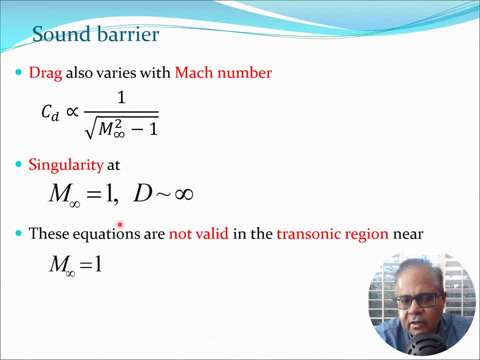 seeing that there is a singularity at m in finity equals 1.. So if I put m in finity equals 1 here, this is going to become 0. And so Cd is going to become infinite. This is something. 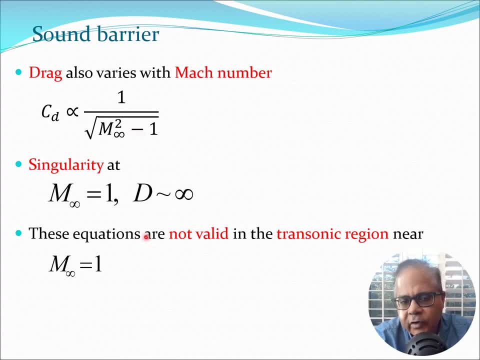 which we can easily see from this equation. Now, one of the facts is, of course, that use of this equation is not actually valid at this m in finity, equal to 1 region. But in the early days, as far as aerodynamics was concerned, people had not yet broken the sound. 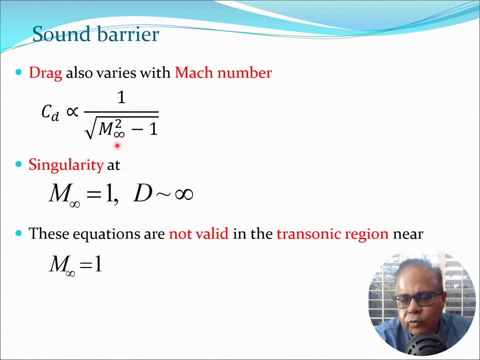 barrier And they used to find that actually the drag would go up as you go faster and faster. So in the transonic region the drag was going up very substantially. So there was some concern that maybe the sound barrier cannot be broken, that it is kind of a physical barrier which 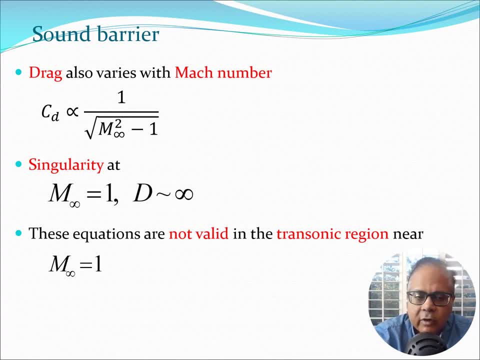 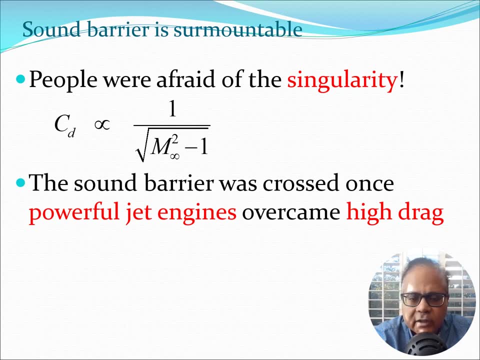 exists because of the laws of physics, And so people had a lot of reputation about this aspect. So people were to some extent afraid of this singularity, And thinking among many people was that maybe, you know, if you tried to do this kind of breaking the sound barrier, the aircraft would. 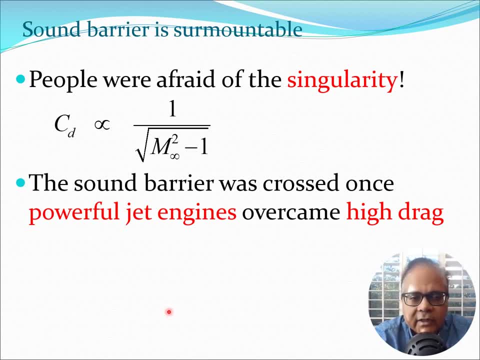 simply break up and, unfortunately, all the pilots and people would all die. So what actually happened is that you could simply break through the sound barrier by having more power, So you have to wait for the jet engines to come up, And once jet engines come came up, people were all 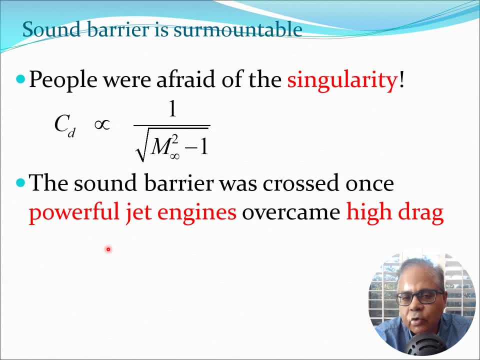 able to sweep the blade, and then they could easily overcome the high drag which was present at this particular regime. so it was not that the singularity could not be crossed. the fact was that this equation itself was not valid at M equal to 1. so these are things we need to keep in mind that very 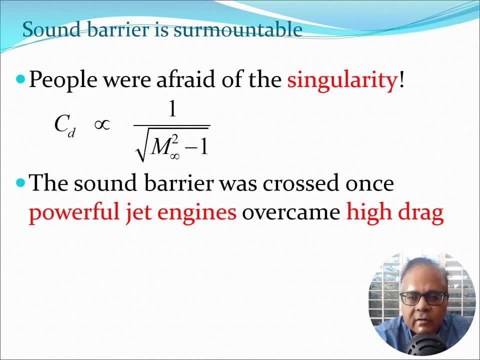 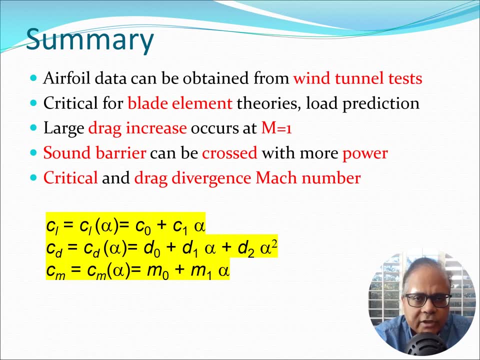 often equations we have, math models we have, may not be valid across all possible regimes. so today's lecture was certainly important because airfoils are the bread and butter of aircraft people and we see that airfoil data can be obtained from wind tunnel tests, which is why wind tunnel tests have been so. 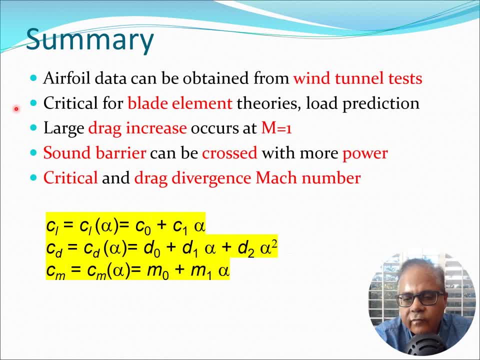 important. fortunately for us, most of the standard airfoils have been tested very thoroughly, and there are books out there which give you a lot of information about the CLCDCM curves, and so you can refer to the link in the description below. Thank you. 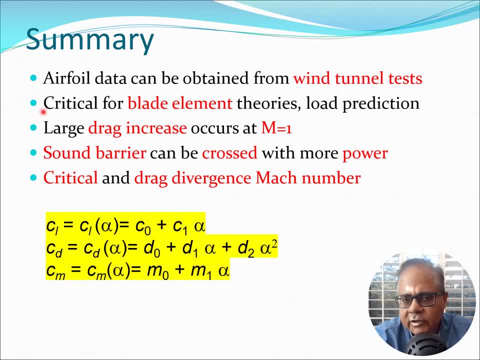 the data from these kind of textbooks, and we also see that these kind of airfoil data is very critical for various theories which are generally known as blade element theories, and these theories essentially consider that you are using a certain piece of the blade in the case of helicopter rotors or wind. 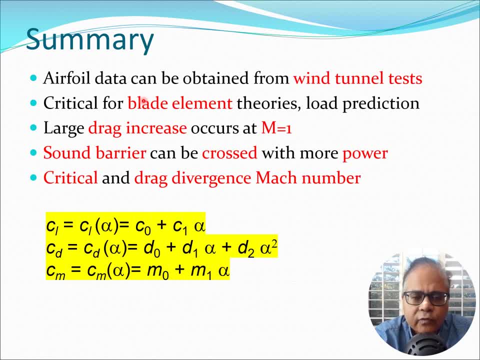 turbine or of the wing in the case of airplanes, and then do various calculations for load prediction based on these airfoil characteristics at that location- CLCD and CM. we also saw that there is a large drag increase taking place at M equals 1 and this is the 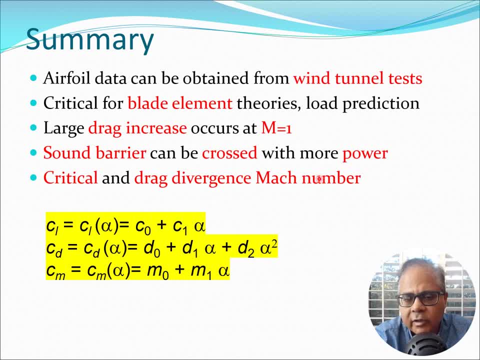 sound barrier, but it can be crossed if you have more power. there's kind of some philosophy behind this also that many times when you face barriers in life, you can probably apply more power and more motivation and cross that barrier. and there's also the important concept of cross-barrier. 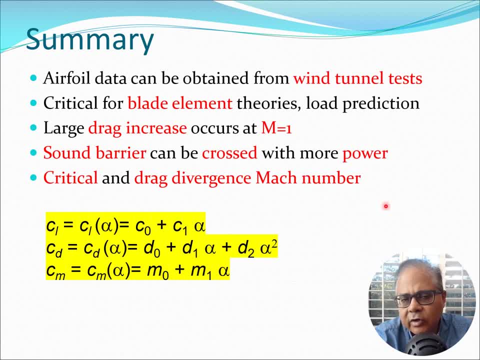 Now let's talk a little bit more about the critical and drag divergence mark number. so these are all related to this variation of CD with respect to the mark number. we are going to discuss that in the detail later. compressibility effects start becoming more important because, as 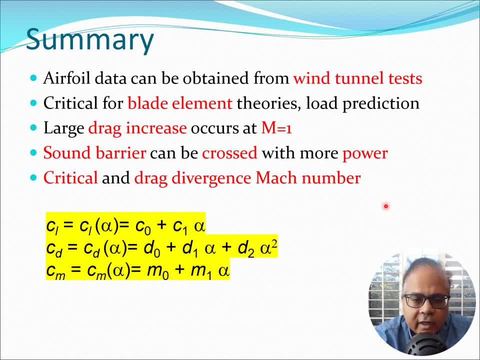 you know, most of the useful aircraft nowadays fly pretty close to the speed of sound, and also some of them even fly faster than the speed of sound and in fact, if you look at most of the jets out there which are flying today, they are flying at speeds which are only slightly below the speed of sound. so these are all. 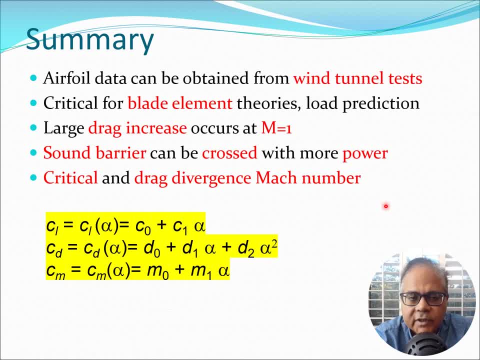 transonic aircraft, and this is the reason why you can fly very long distances nowadays, for example, between Bangalore and San Francisco in one direct flight. so these things have become possible because of the advances in aerospace engineering. Now let's talk about the technical aspects of the airfoil that we are going to 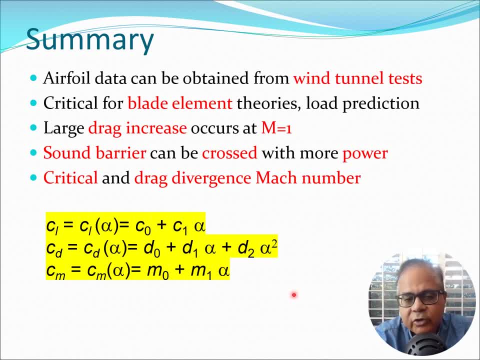 discuss today. First of all, we are going to talk about the technical aspects of the airfoil. First of all, we are going to talk about the technical aspects of the airfoil. First of all, we are going to talk about the technical aspects of the airfoil. 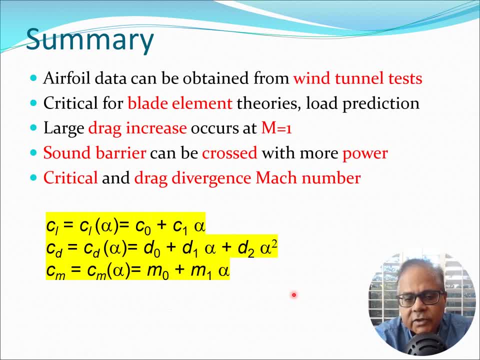 So just to summarize again the simple math models which we discussed today, CL was C0 plus C1. alpha C1 is the lift curve slope, CD is D0 plus D1 alpha plus D2. alpha square CM is M0 plus M1 alpha. and always remember that CD must always be.